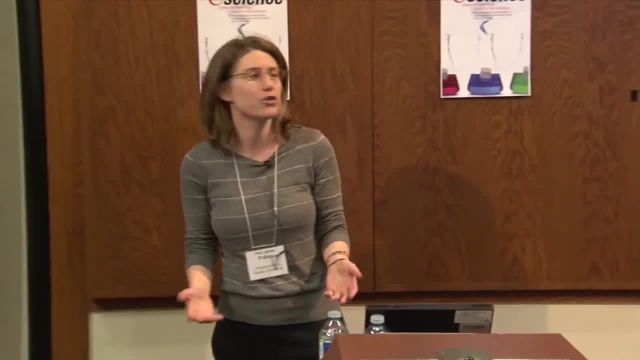 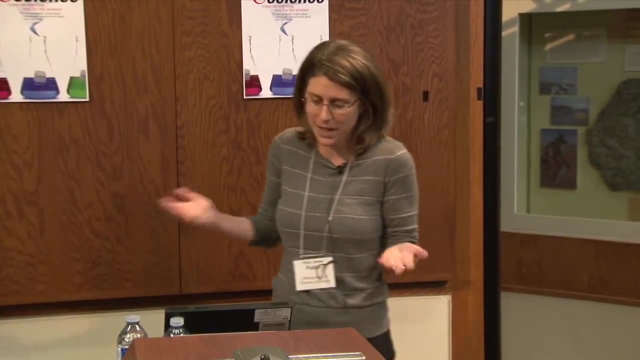 there's vertical transport in the ocean which can bring those nutrients back up to the sunlit surface ocean, without which the ocean would be a stagnant and lifeless abyss. We'd have a stagnant and lifeless abyss in the ocean. So there's just one more problem, which is that the oceans heated from above by 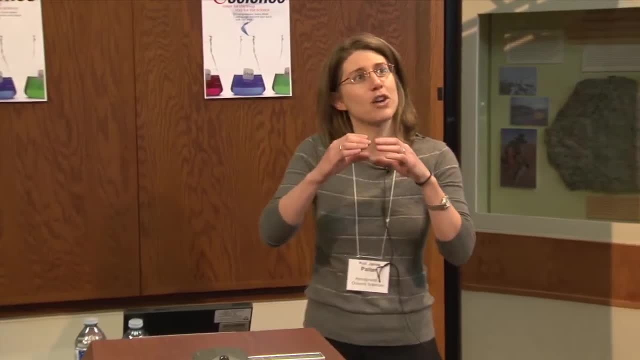 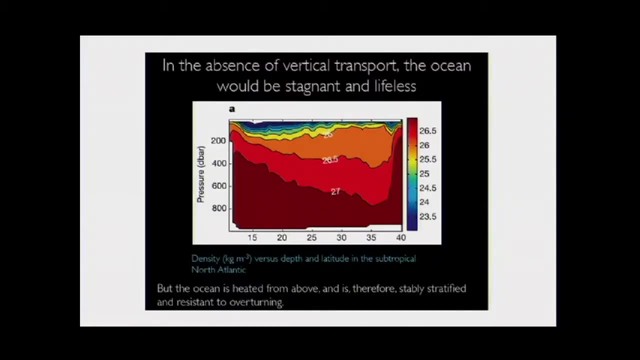 sunlight coming in from the surface. so it's therefore stably stratified, which means that there's less dense water sitting on more dense water and there, and also very resistant to vertical transport, because you have to overcome that buoyancy effect of having light water on dense water. So this is the same. 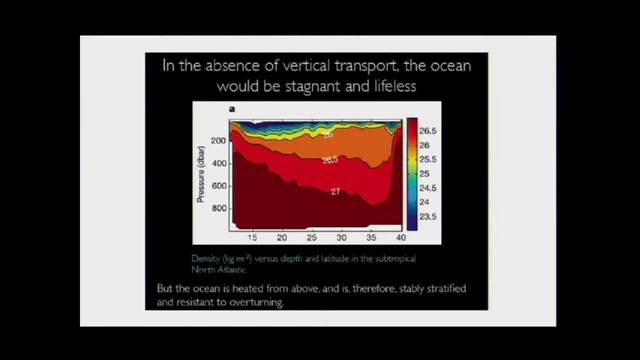 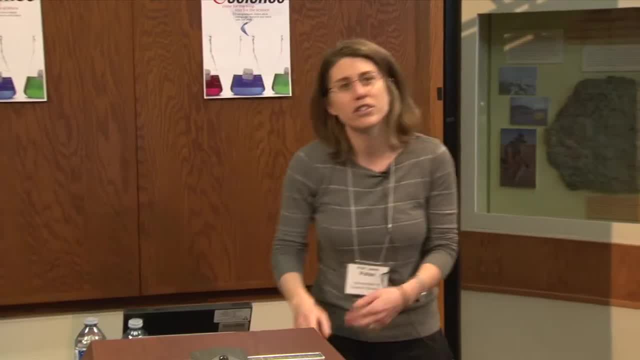 slice through the subtropical North Atlantic showing the density structure and you can see the light. the blue colors are light density and the red colors are heavy density. we have light on heavy. So my research examines these physical processes that shape the living ocean. So how do we reunite, for instance, how do we reunite? 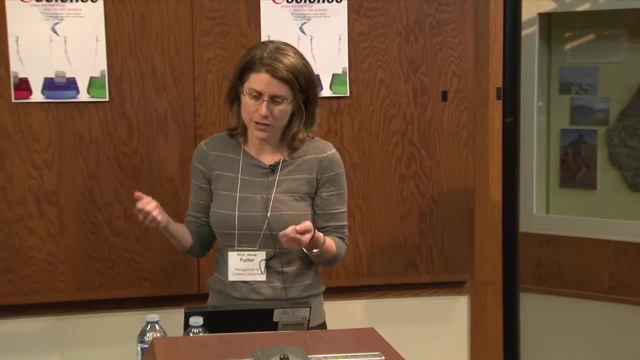 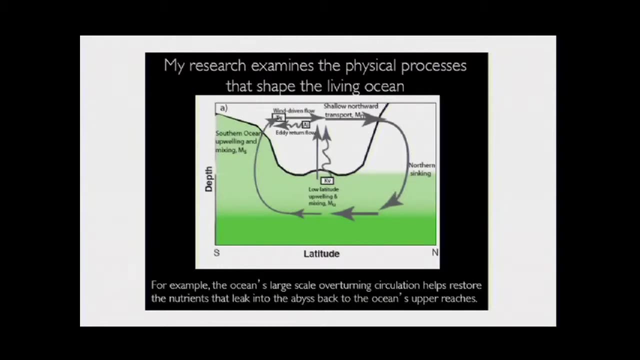 the nutrients at depth with the photosynthesizers at the surface. One thing I've looked at, for example, is the oceans large-scale overturning circulation. So there's- this is a schematic showing the northward transport of light waters at the surface ocean which sink at high northern. 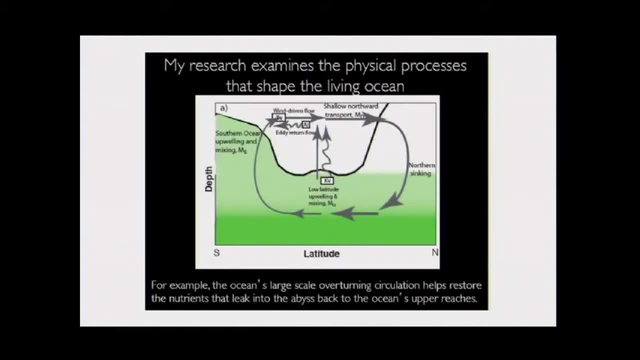 latitudes flow in the deep ocean back to the southern ocean, the Antarctic circumpolar current that encircles the earth at the low southern ocean, at the high latitudes in the south southern hemisphere, and come back up. So this overturning cell in the ocean helps over 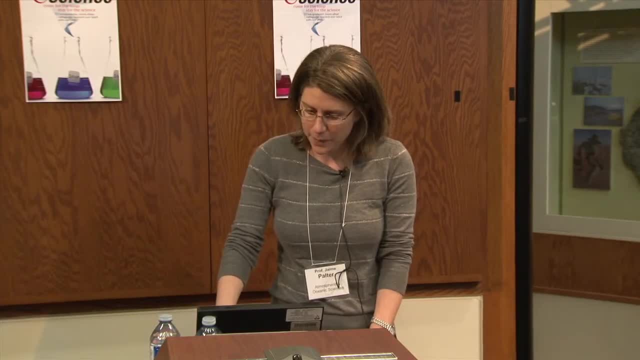 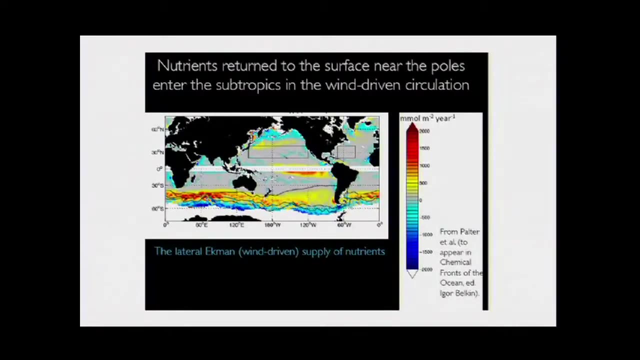 long time scales, restore those nutrients that leak to the abyss. Finally, because those are processes are important. at high latitudes, this overturning happens to bring the nutrients up, particularly in the Southern Ocean. This map shows how the nutrients then are transferred horizontally in the wind driven. 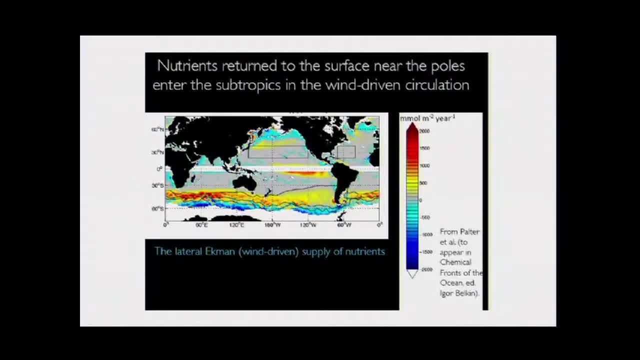 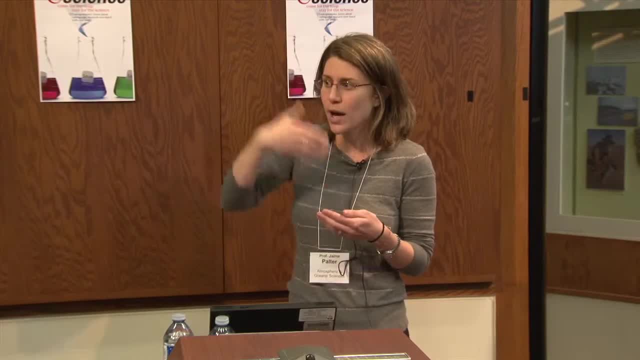 transport from the high latitude ocean. So in the blue colors at the very southern extent of this map show the loss of nutrients from the Southern Ocean and their transport. those red colors their supply to the subtropical gyres. So that's one way that these nutrients are restored to the subtropics. Thank you.